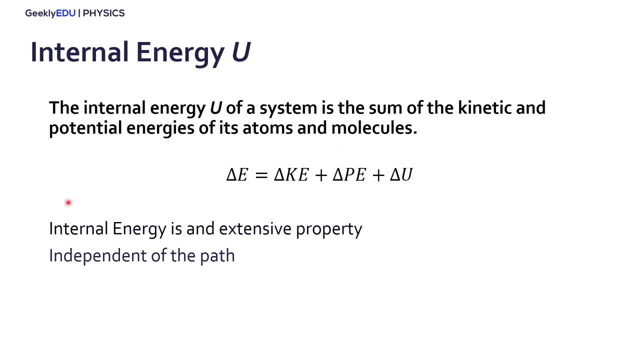 okay, well, we need to know is that internal energy is an extensive property, so it depends on the mass of the system, and also that it's independent of the path from the system, so it independence of the path, of the path, if the system is going from its initial state to its final state. 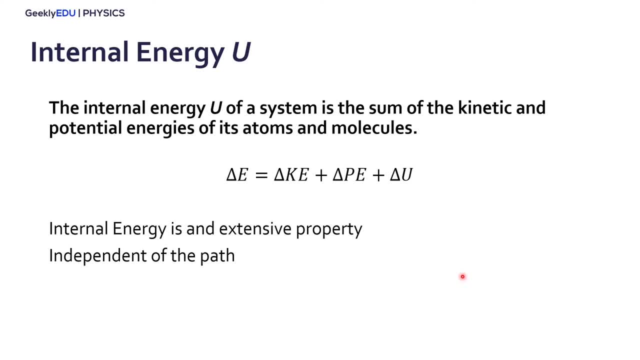 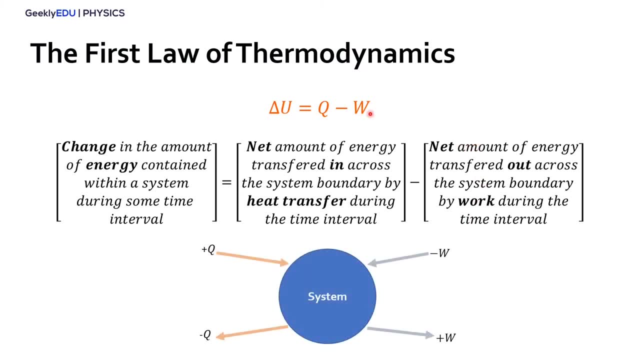 it doesn't matter the in between these two states. okay, all right. so the first law of thermodynamics tells us that the change in the amount of energy contained within the system during some time interval equals the net amount of energy transferred in across the system boundary by heat transfer during the time interval. 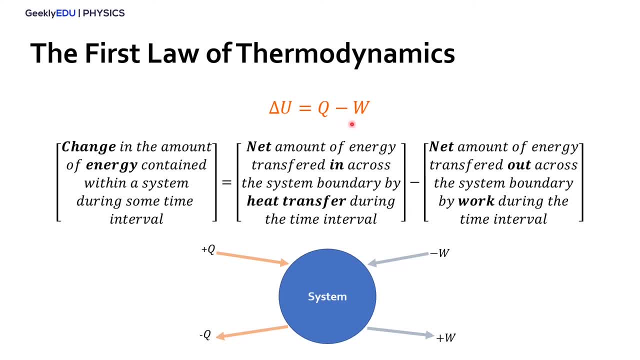 minus the net amount of energy transferred out across the system boundary by work during the time interval. so we have a system here. we have heat transferred in and out and work done by the system or in the system. okay, so by convention we say that the heat transfer 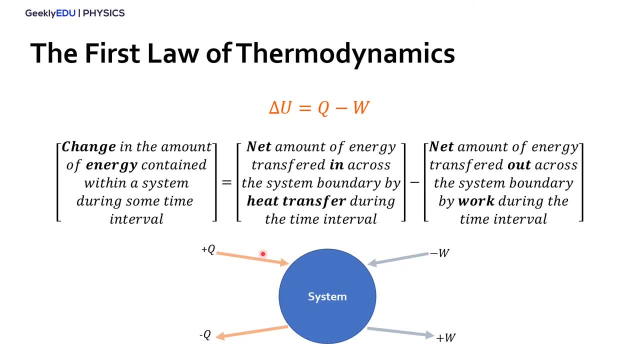 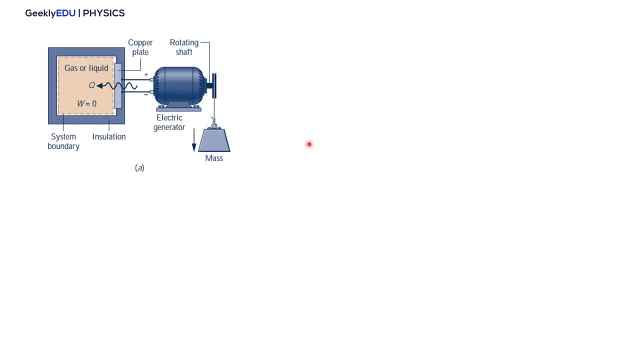 in the system, okay, is positive and the heat transferred out of the system is negative. for work is the opposite, right? okay. it's very important when dealing with this thermodynamic problems to define the system boundary. okay. for example, in this situation, here a, if we define our system boundary as inside this box, here this: 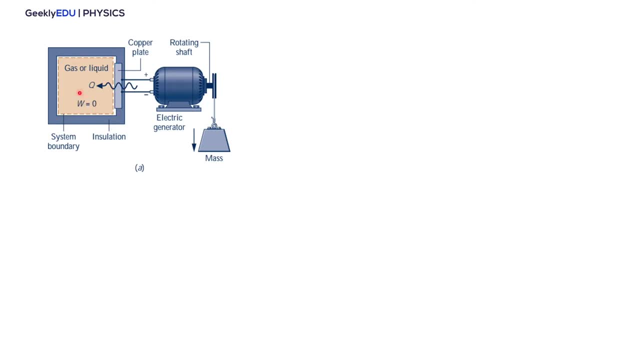 insulated box, we don't have any work, right, nothing's happening here through this. there's no work going in or out the boundary, but we have heat transferred from outside to the inside of the boundary, right, okay. however, if we set the system boundary as outside the insulated box, well, it's. 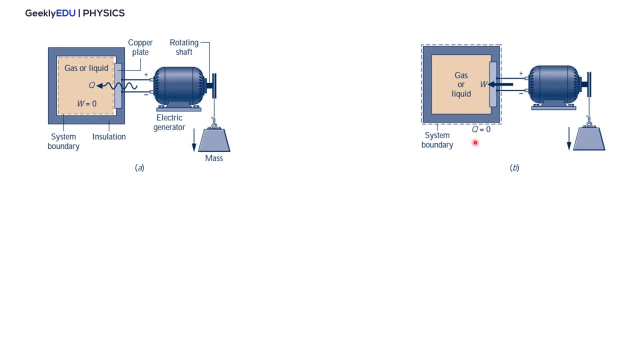 insulated, so we don't have any heat transfers here. but we have electricity that is moving this weight, is lifting this weight right, so it's work. so in this case we have work but no heat transferring. also, if we set the system boundary outside everything here, well, in this case we don't have any heat being. 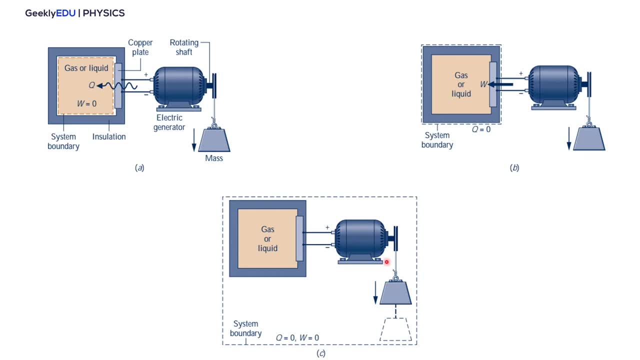 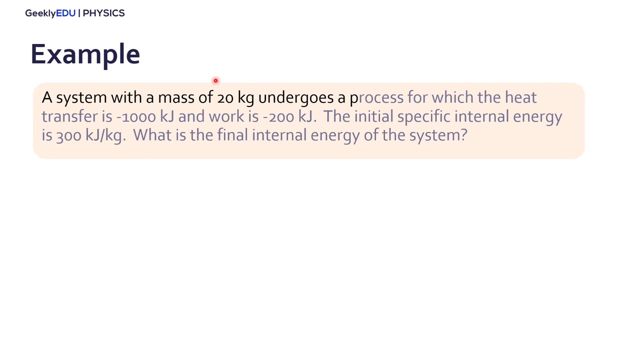 transferred through the boundaries nor work done through the boundaries. so it's very important when solving thermodynamic problems to set your system boundary in a way that you're going to solve the problem all right. all right, so let's go through this example here. we have a system with a mass of 20. 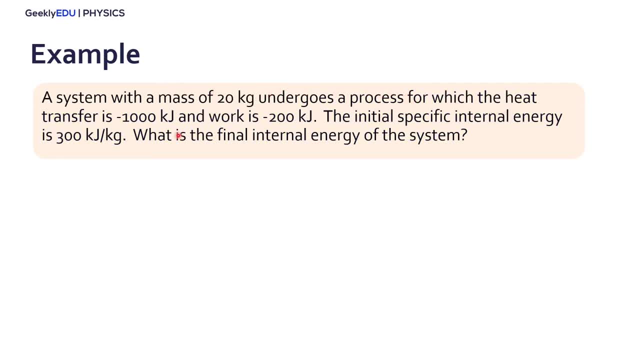 kilograms that undergoes a process for which the heat transfer is negative a thousand kilojoules and work is negative 200 kilojoules. so the initial specific internal energy is 300 kilojoules per kilogram. so what is the final internal 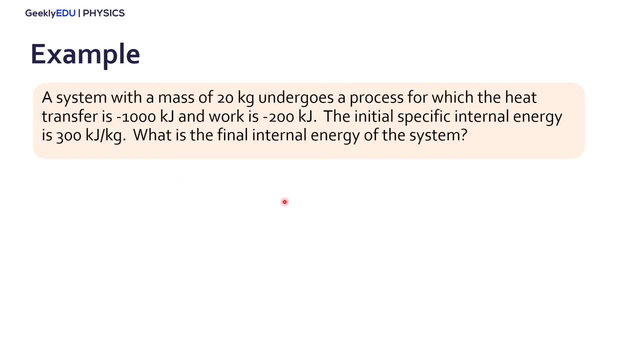 energy of the system. so let's sketch the system here. the problem: we have a system of 20 kilograms. the initial internal energy, specific internal energy- is 300 kilojoules per kilogram and we have two negative energies here. so we have a negative heat transfer, which means it's going in the system. 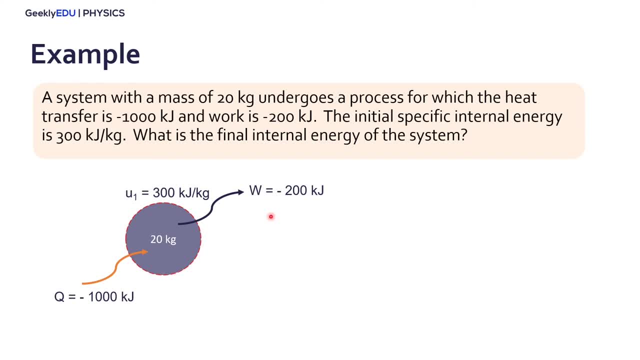 from outside to the inside and negative work, which means it's going from this system to the outside of the system. okay, it's very important to know the signs here and understand where the energies are going. so let's apply the first law of thermodynamics. we have the variation. 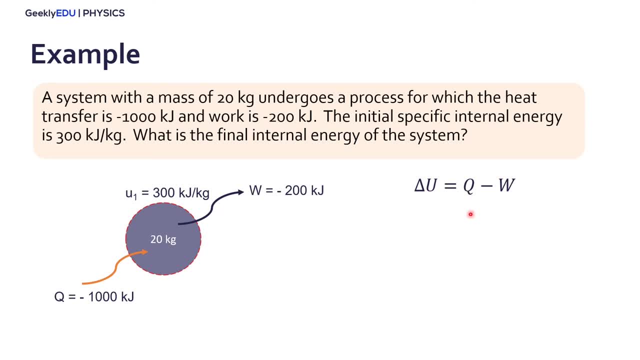 in internal energy is the heat transferred minus the work. so we know that the specific internal energy, we can multiply it by its mass right, so we have the heat transfer minus the work. so we know that the specific internal energy, we can multiply it by its mass right, so we have the.